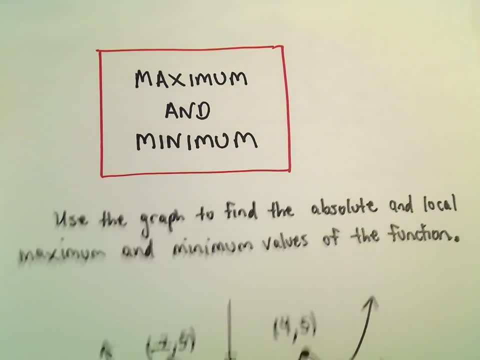 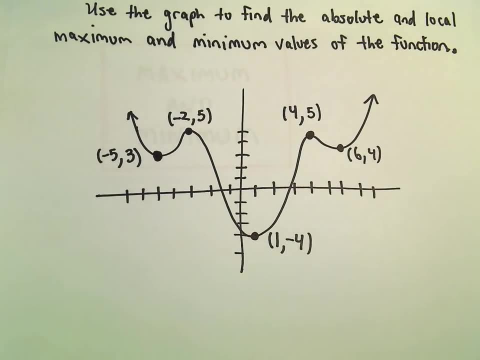 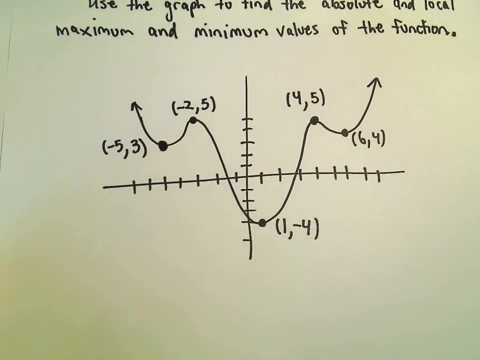 Alright, here we've got an example where we're going to use the graph to find the absolute and local maximum and minimum values. So absolute maximum and minimums and also local maximum and minimums. Oftentimes people just give the y values, so we can kind of use both notations here. 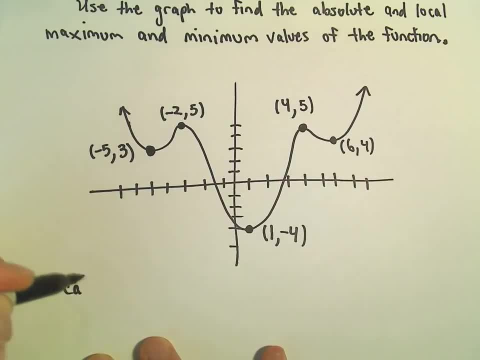 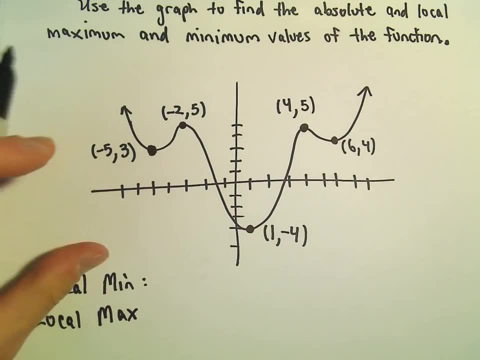 So if we want to figure out sort of the local minimums and also sort of the local maximum values, well again, I just kind of imagine I'm looking sort of at a mountain range off in the distance, you know, obviously kind of a weird mountain range because it keeps going forever. 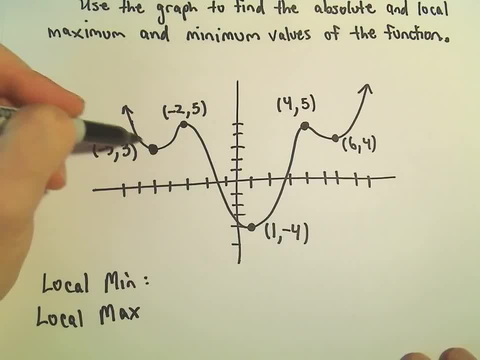 but if we're looking for local minimums, I'm kind of looking at, you know sort of imagining, like you know kind of looking at the valley of my mountain range, sort of a you know just where it bottoms out. 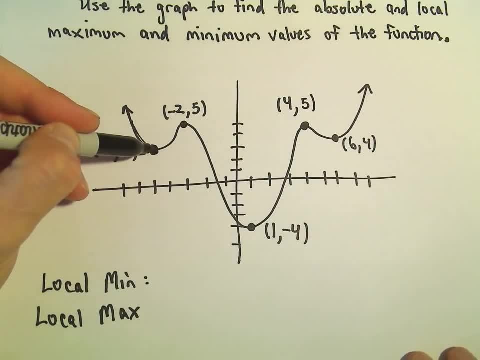 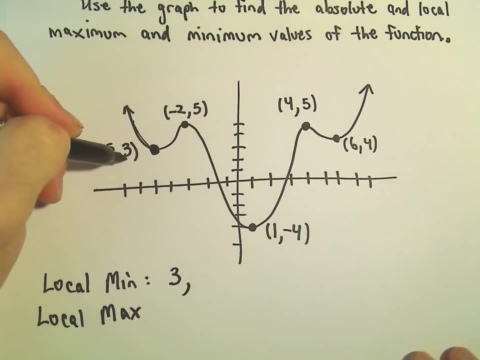 So at this point we're going to use the graph to find the absolute and minimum values. So at this point we would say we have a local minimum and oftentimes people will just specify the y value. So we could say the y value of 3 corresponds to a local minimum. 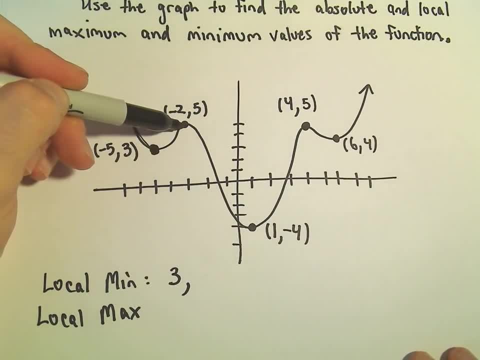 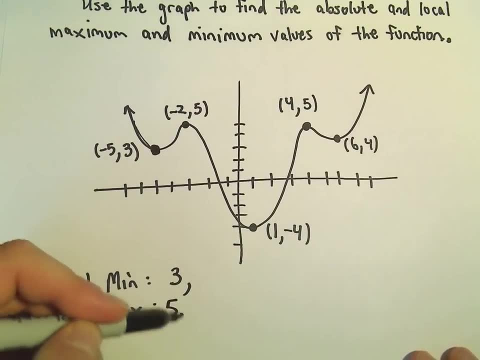 Well, let's see when we get to this point. notice this is kind of like a little top of a hill- That would be considered a local maximum. So we could say we have a local maximum at the y value of 5.. 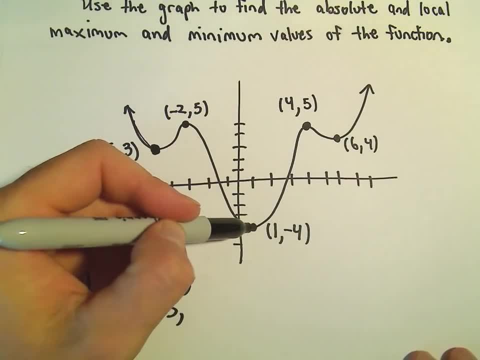 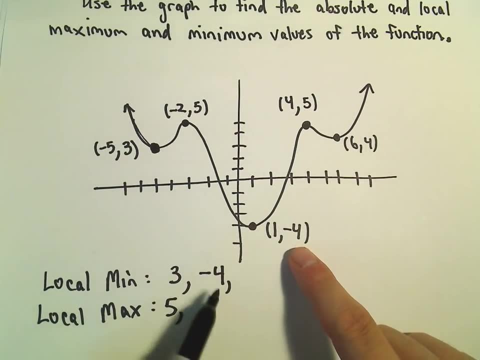 Again as we go down it kind of bottoms out here at this point. So again, that would be a local minimum. So we have a local minimum at the y value of Here. at the point we kind of have the, you know, the little top of the hill. 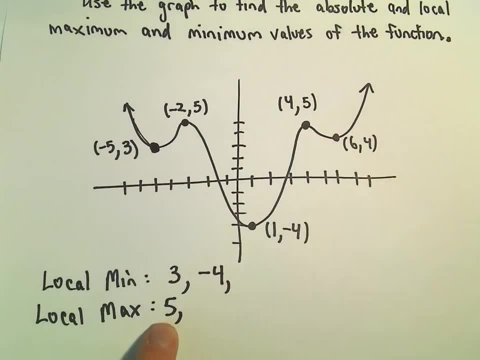 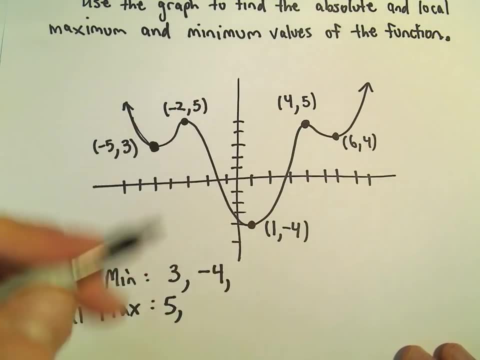 So again, 5 would correspond to a local maximum value. but we've already got it listed so we don't have to list it again And again. at this point you're at the bottom, So we could say at: y equals 4, there's a local minimum. 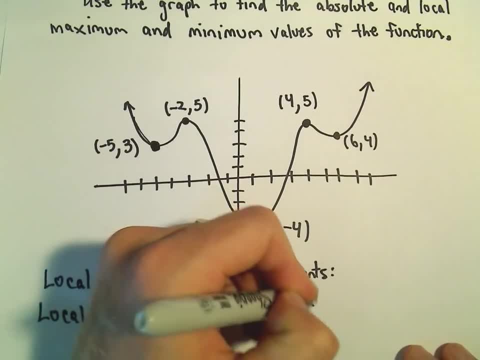 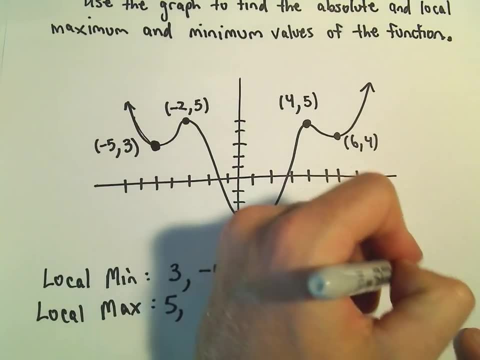 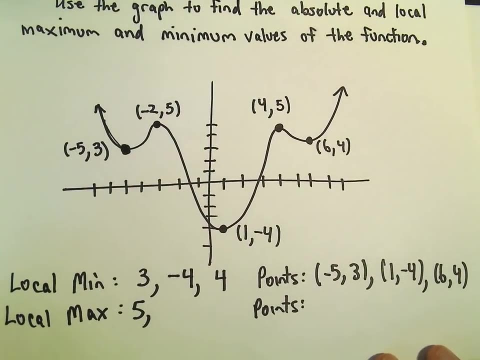 If you actually want to specify, you know the points. obviously you just do the same thing. So you could say: you have a local minimum at at the point and also at the point, Squeeze that guy back in there.